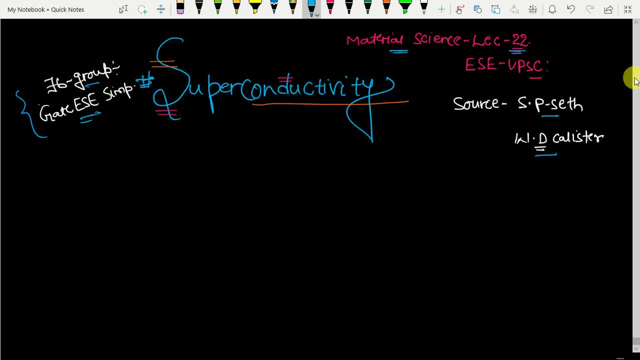 let me introduce you the term superconductivity. What is superconductivity? It is a state of material science, engineering. It is a state of material science, engineering. It is a state of material in which it has zero resistivity. That is. superconductivity is the concept in which the 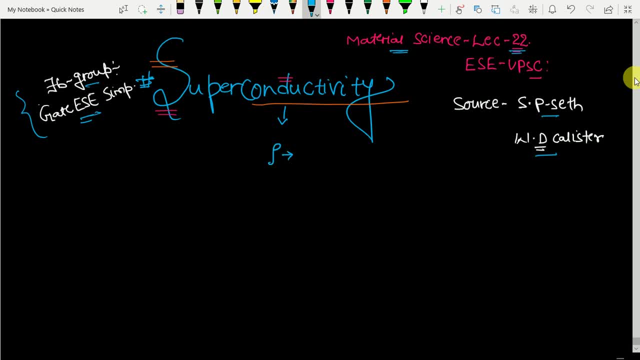 material has resistivity is defined as: rho has zero resistivity. This is a super. you can say that this is a highly ideal condition, but superconductivity concept is based on this only. That is, for a superconductive material, the resistivity of that material has zero is zero. 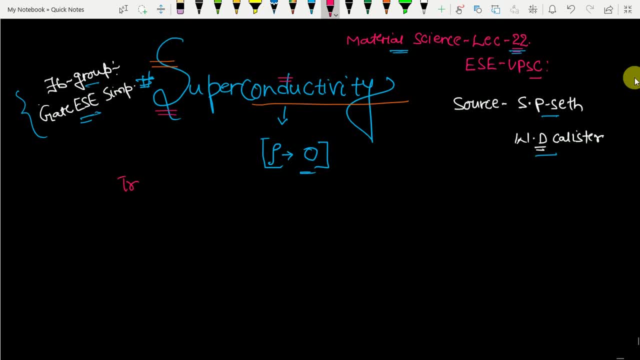 Now there is a term known as transition temperature, Transition temperature, The critical temperature. it is a temperature. You can say that it is a temperature or the critical temperature at which there is a change of state, from superconducting state to normal state or vice versa. That is, let's say, transition temperature is Tc, It is a state. 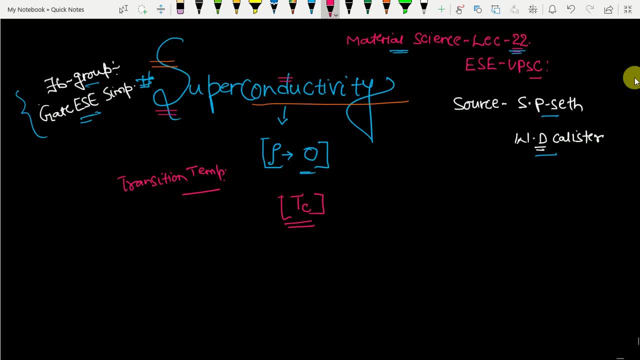 This is a boundary state from which the critical temperature- this is a critical temperature at which there is a change of state, That is, the conductivity of that material- will change its states. from that there will be some change in state from superconducting state to normal state or vice versa- is known as transition temperature. 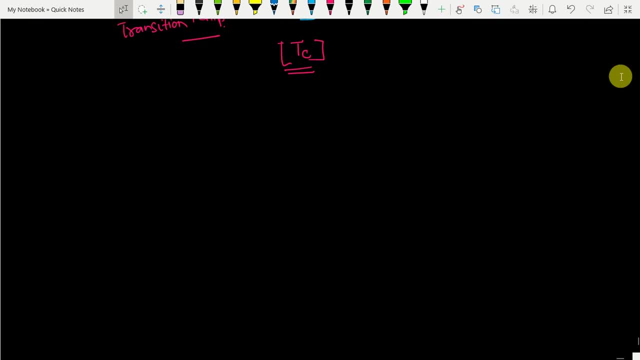 Now let me show you how. If you will plot resistivity versus the temperature of a material, then the plot you will get is like this: That is at transition temperature, TC, and after that it will change its normal state. like this: It's a state line, That is, this will represent normal state. 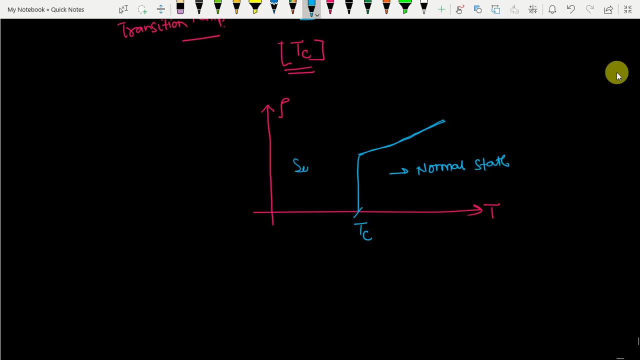 And this is superconducting state. superconducting state. Now let me move further. Now let me explain you a term: mizner effect. This is the important concept: mizner effect. You have to remember, or you have to keep in your mind, because you can expect question related to this mizner effect. 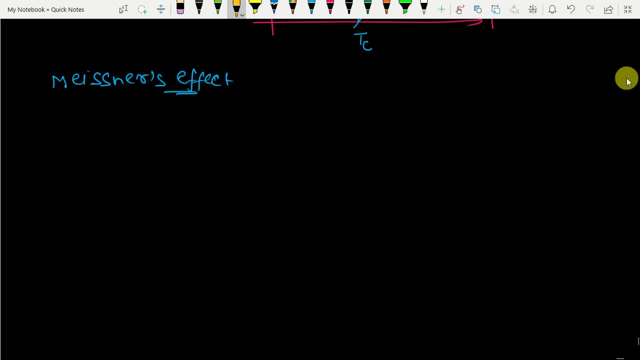 It means, according to mizner effect, the repulsion of magnetic flux Line, that is, repulsion. repulsions of magnetic flux lines from the interior of a piece of a semiconductor material as the material undergoes transition to the superconducting state, is known as mizner effect. 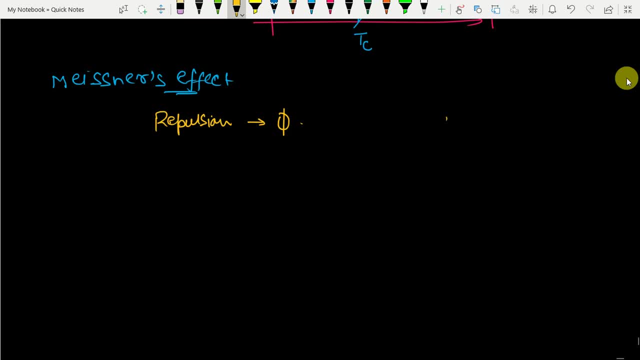 That is, whenever we will take. let's take a normal material and if we have applied a magnetic field, you can say that B is the magnetic field applied across this material and what we will observe is that the magnetic field is applied across this material. So magnetic field passes through in the normal, in through the material in the normal state. 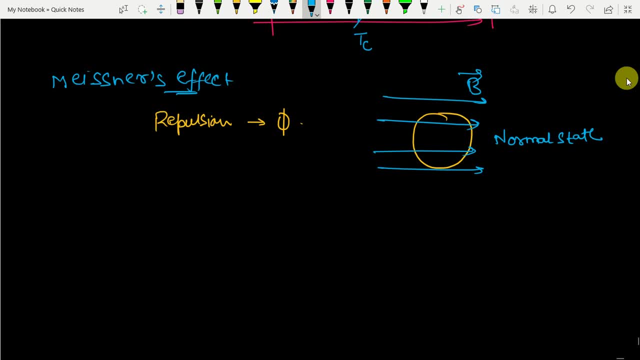 It means what will happen in the normal state that we take material, that we take in the normal state Under the normal condition and normal state across that superconducting material, the magnetic lines of forces pass through this normal state. What do you mean by the term normal? Normal state means that temperature is greater than TC. that is critical temperature means if we take more temperature so superconductor will behave like a normal state. 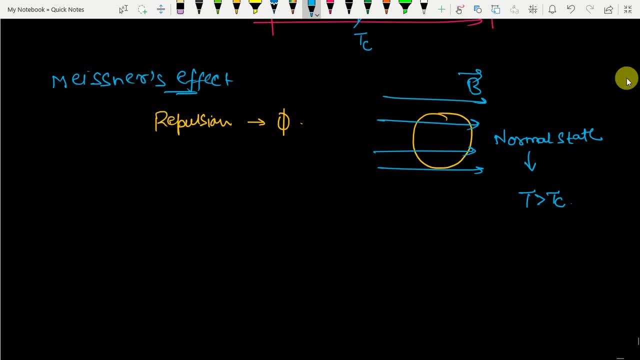 What will be the meaning with this term normal state? All this can be красh Because of the one thing: in the way you take this, material's temperature is greater than TC. it will remain spirit and form state in the form of normal state. now, when, when t is less than tc, that is, when the temperature is. 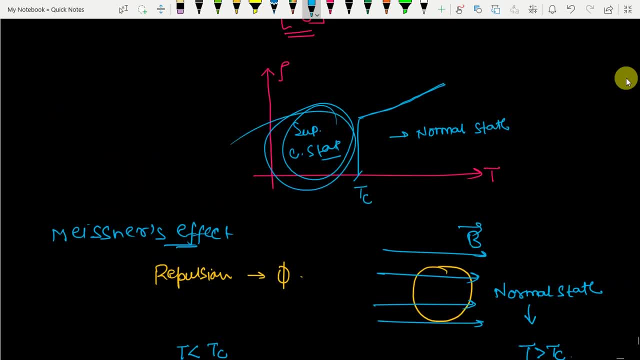 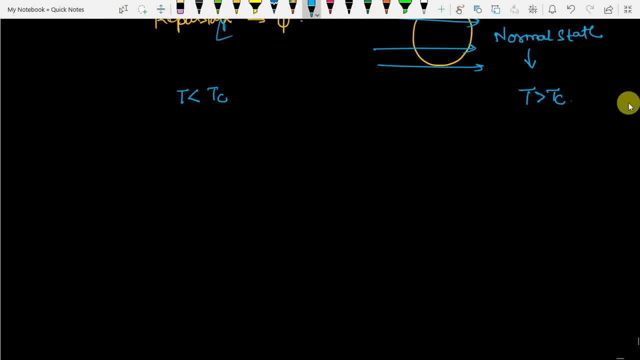 less than critical temperature. that is, i am talking about this zone, this is zone of normal state and i i am talking about this. that is the when t is less than tc. in this case, when, when we expose the superconducting material- superconducting material- into a magnetic field, you can say that 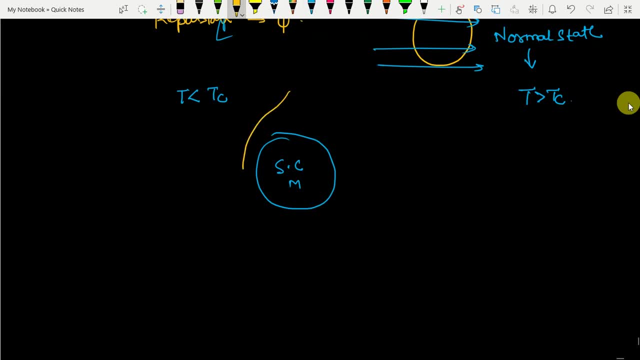 then there will be repulsion of magnetic lines, of forces like this, like this. you can remember. this is the like, the same. in case of diamagnetic material we applied the external magnetic field like this: it is: the condition of t is less than tc, that is superconducting state. so you can say: 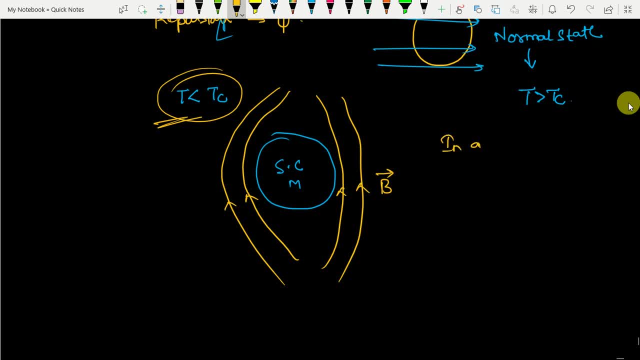 that, just like as diamagnetic material in a super, in a superconductor, you can say that inside the superconducting material, the net magnetic field, magnetic flux density is zero. but as we know that vector b, that is, magnetic flux density, is equals to mu naught h plus m. 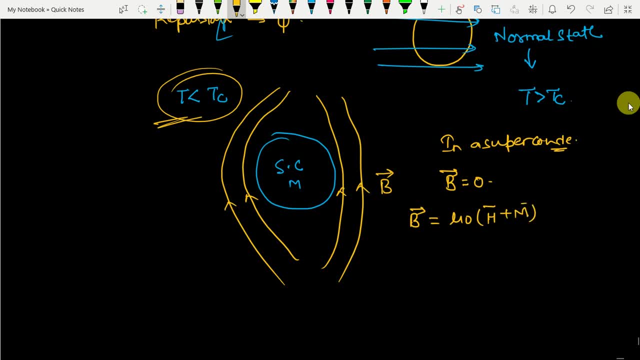 where h is magnetic field intensity. now, in this case, as b equals to zero, replacing b as equals to zero equals to mu naught h plus m. you can write it like this, so from here you can, you will get that m equals to minus h. okay, that is m by h ratio. that is the susceptibility. 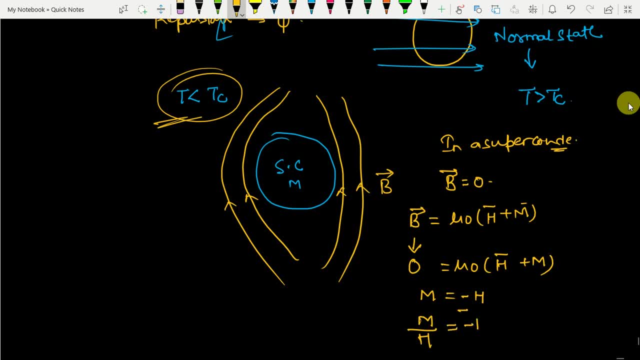 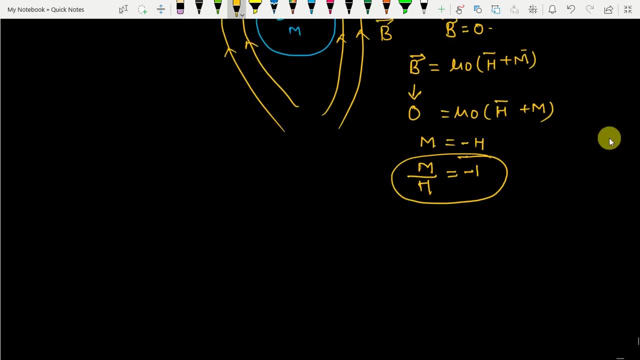 is negative, that is, it will repel the magnetic lines of forces through them. so you can say that from this we got the relation mu: r minus 1 equals to minus 1. we can write, as i have already explained this thing in my magnetic material concept, so you: 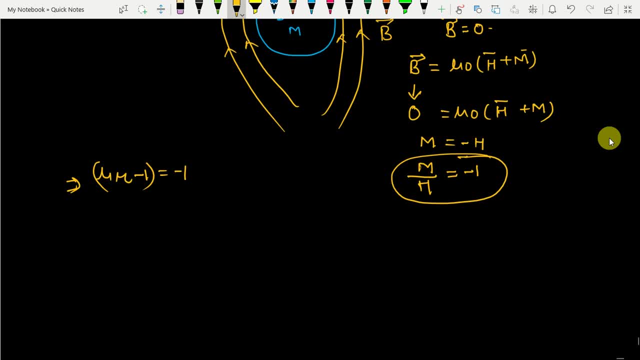 you can refer there. if i haven't, if you haven't gone, went through them. so mu r minus 1 equals to minus 1. from this we can say that mu r minus 1 equals to minus 1, equals to minus 1, equals to minus 1. 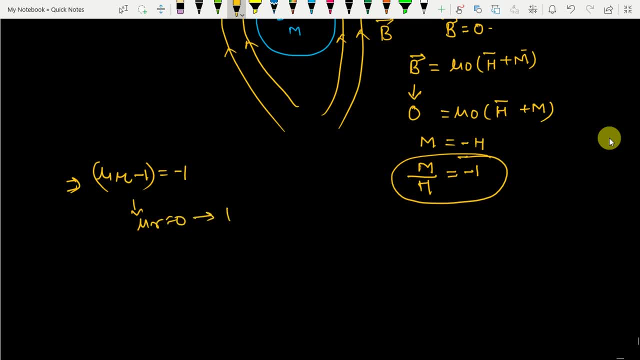 you can get mu r equals to zero. that is, this is the condition of perfect diamagnetism. if you remember the concept, i have already cleared the these points in my previous lectures. that is, perfect diamagnetism is an independent property of superconductor. that is, you can remember this. 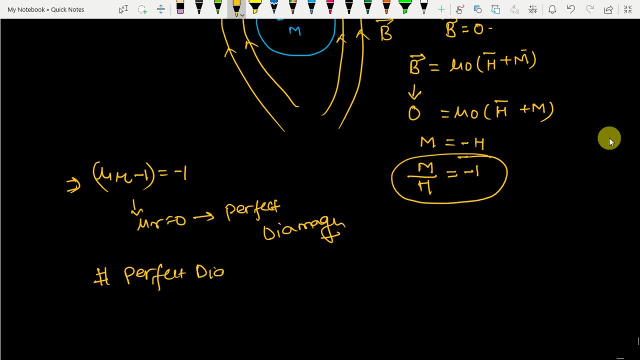 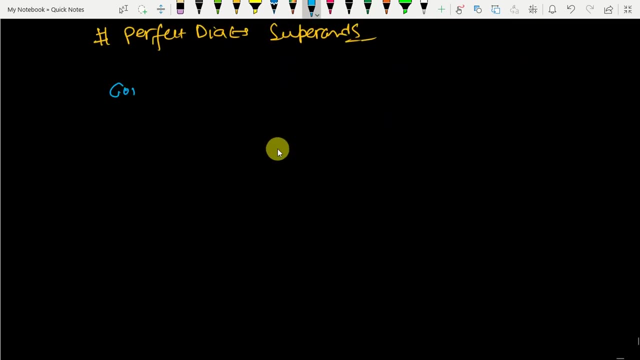 point. perfect diamagnetism is the independent property of superconductor superconductors. now moving further, there are some condition for superconductivity. let me explain you that conditions, that is, conditions for superconductivity. the conductivity is like that. resistivity must be equals to zero. condition number one: 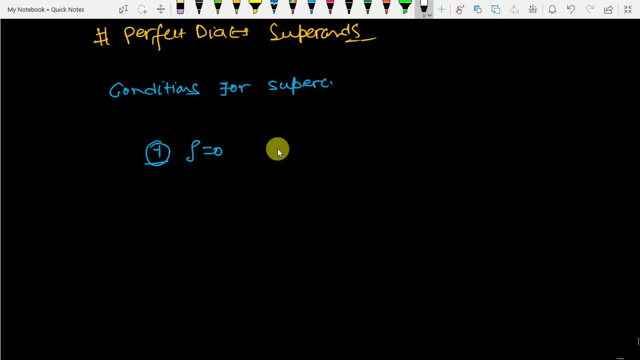 you have to remember these points because you can expect question related to these points, either in case of multiple choice options, or you can expect question related to these points, or you can also expect a question related to them in case of assertion reason type question. this is very much important. now the second point. the second condition for superconductivity is it. 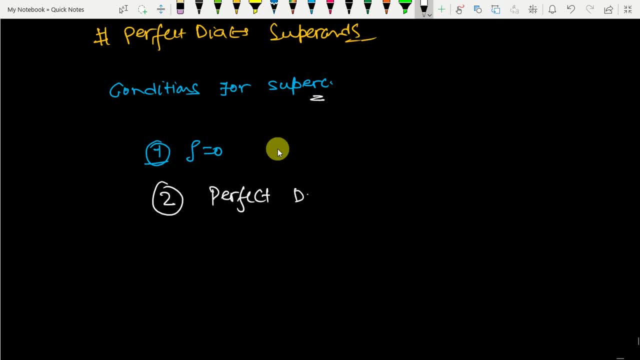 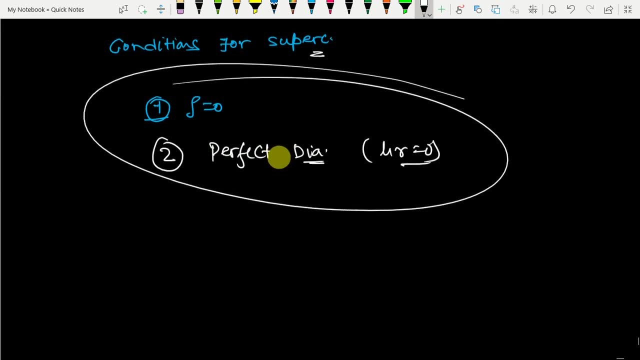 should be perfect. diamagnetization- diamagnetic, that is mu r of material equals to zero. these two are the conditions for superconductivity of that material. now let me start superconductors, so you can explain superconductors as like that. these are the materials which exhibit resistivity. 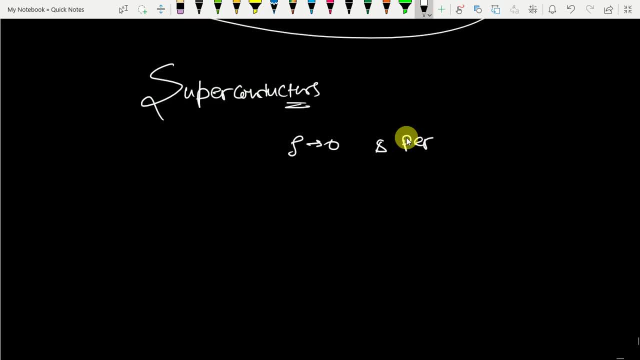 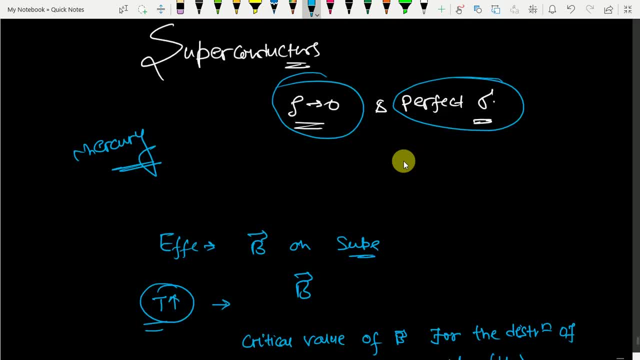 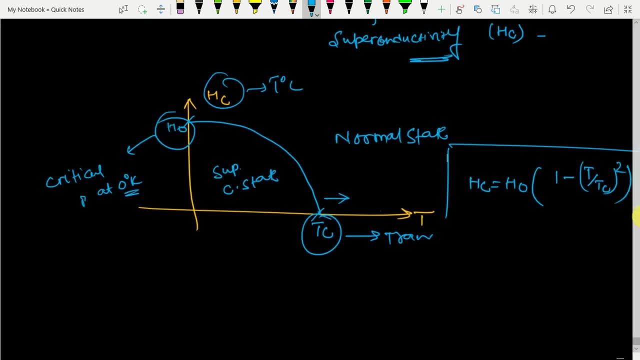 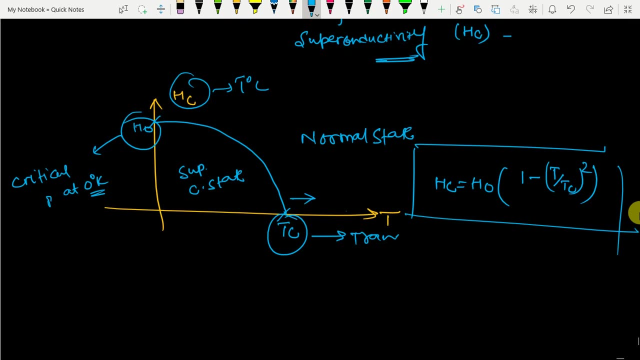 whole square, this relation you have to remember, and i have already explained. i have already explained what is hc, i have already explained what is hc and what is h naught. that is, hc is the critical magnetic field at t temperature, t naught degree cells, kelvin. h naught is the critical magnetic field at zero. 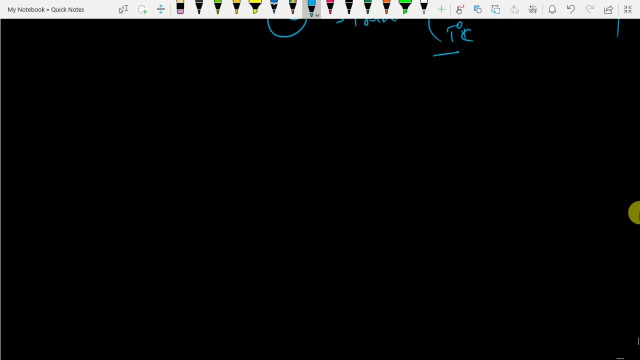 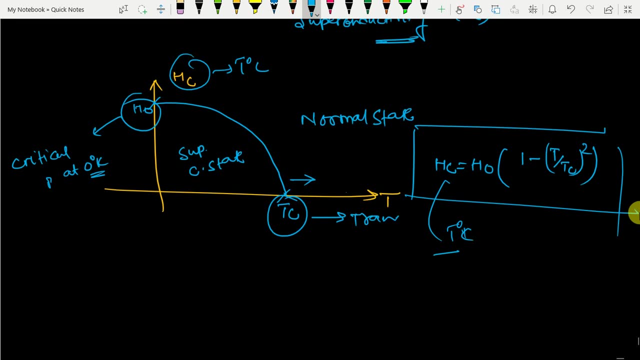 degree kelvin htc is the transition temperature now moving further. so you have to remember these points because these you can expect question related to these terms. you can easily expect question related to these terms because they used to ask: and these are the most important topic for: 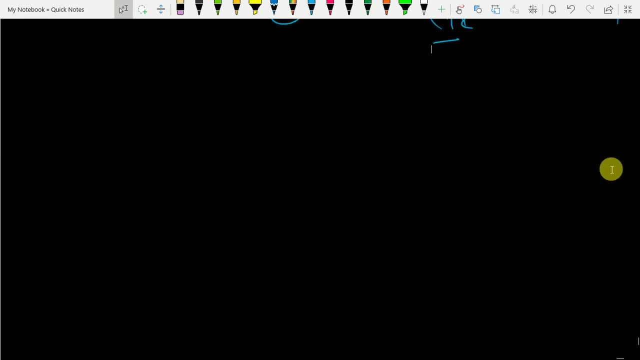 so from the superconductivity topic. now the second important point is: let me explain you: sils b is a rule, sils b is rule. kindly be focused, because this rule, this is very much important rule. according to sils b rule, the magnetic field which causes the superconductor to be, come normal from a superconducting state, that is. 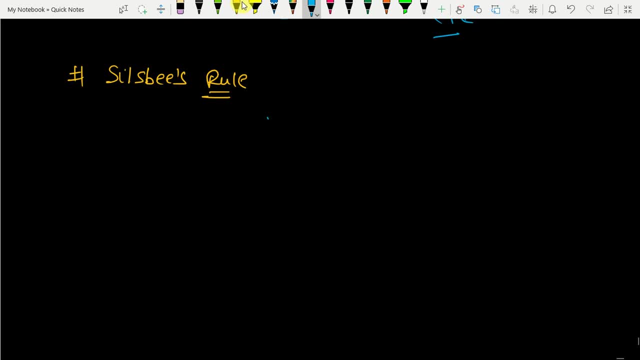 so this is magnetic field. the magnetic field which causes a superconductor to become normal from a superconducting state is not necessarily an external applied field. what we have applied, an extra external magnetic field, will changes the superconductivity from the, from the superficial or 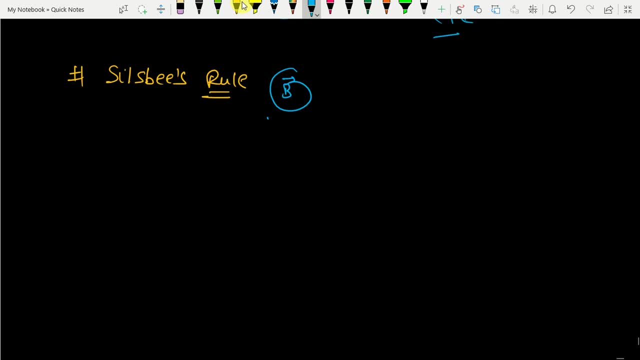 superconductivity state to the normal state but it may arise at an electric current flow. in the current it may, it can also cause that is, the variation or the or the transition of superconducting material from superconductivity state to the normal state will also cause, because of the current applied across that. 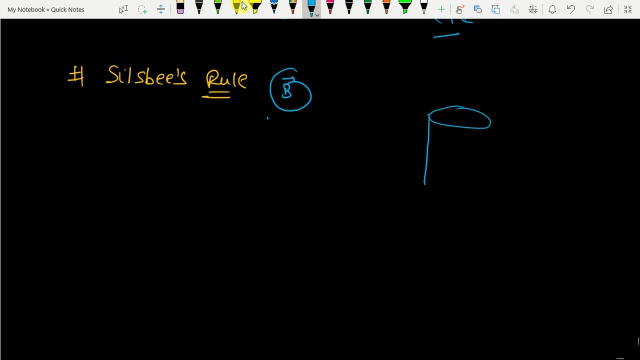 conductor. let's take- i am taking- a conductor, cylindrical conductor like this. okay, now let's say that i is the current flowing across this. i'm not that much good at this- is the radius of this conducting this cylindrical wire. let's say now, so according to amperes law, as we know that cyclic integral h dot dl will be equals to: i enclosed. 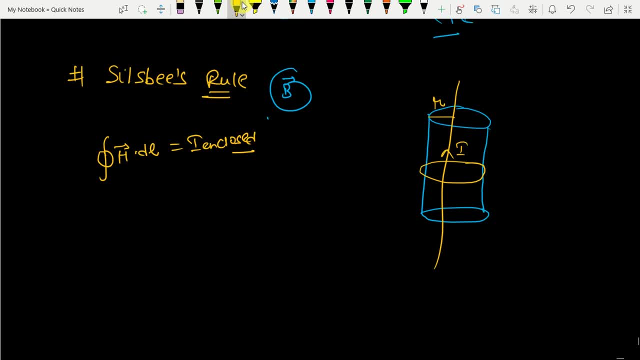 from amperes circuit law, as we know that. so from there you can conclude that hc, that is the critical magnetic field intensity into 2 pi r, r is the radius of that cylindrical conductor- is equals to ic. from here you can write that ic equals to. 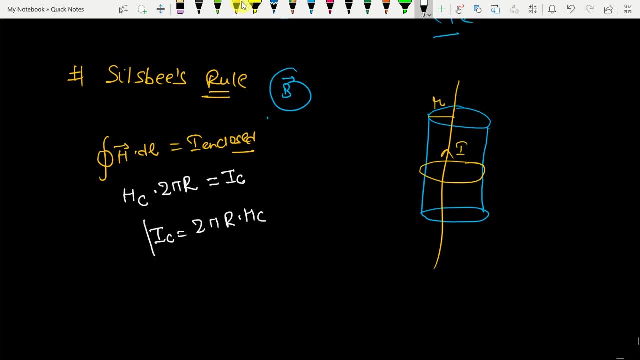 2 pi r into hc. this is the important relation you have to remember. this is known as ic, is known as critical current, critical current. now we have calculated from the silsvi rule the value of critical current, so you can also calculate the value of critical current density. 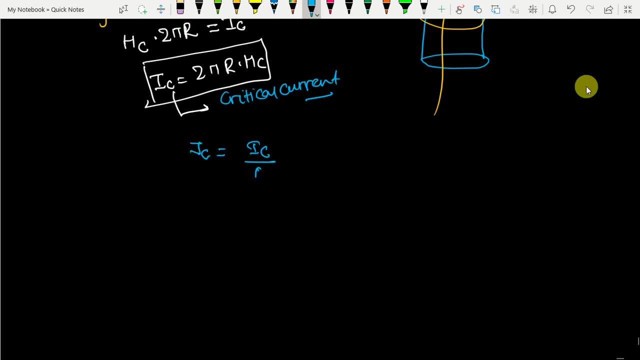 that is jc. jc will be equals to ic by a. that is, this is critical- current density. critical current density ic is what? 2 pi r into hc, as i have calculated above, divided by area, is what area is simply pi r square. so this r and this r cancel this pi and this pi cancel so you can write it as jc. that is critical. 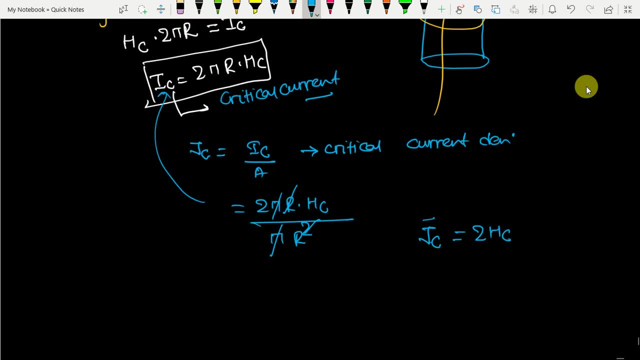 current density will be equal to critical current density, that is, jc, that is, critical current density with, will be equals to 2 hc upon r. this is the important relation and you have to remember it because you can expect question related to critical current density and current critical. 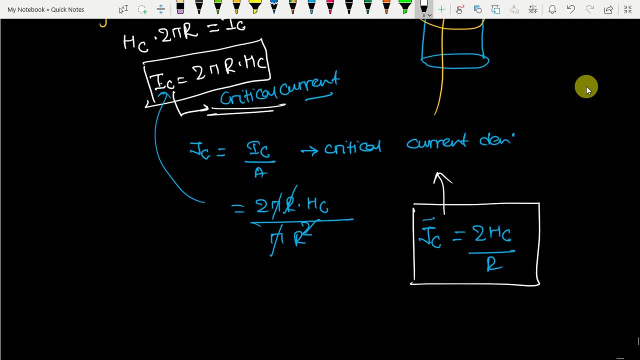 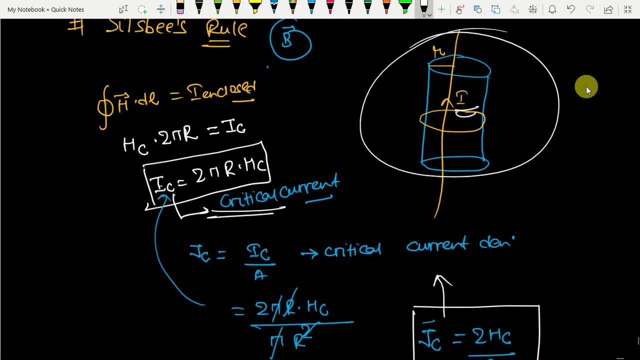 current concept, that is, if a superconducting material carries a current. let's explain this: if a superconducting material carries a current i such that the magnetic field which it produces is equal to critical magnetic field, then superconductivity disappears. that is superconductivity. 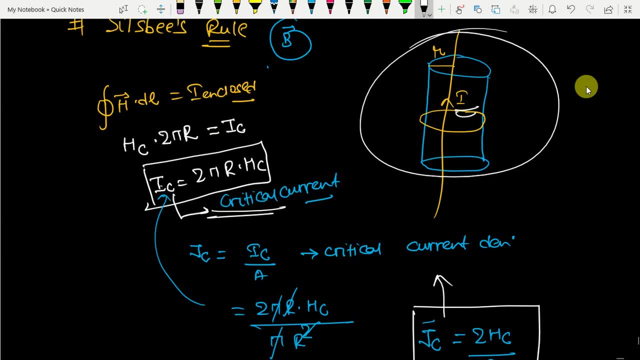 disappears and formed barrier, lower barrier. it husbands also, of course, and it also capaz of conductingjanetic material. so sorry, we get it now. so, for example, if say here, if okay, so here, in case of it sells v, sells v, tells us, according to csp rule, you cannot only transform. 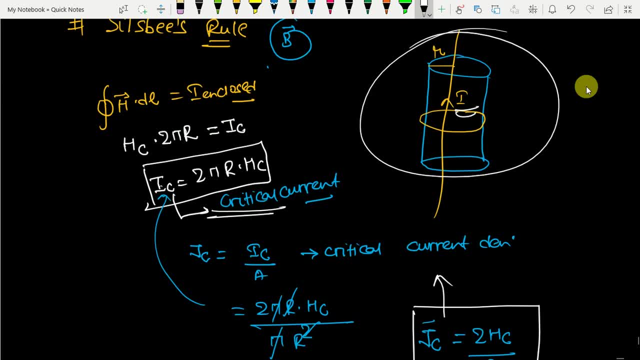 the superconductivity of material, that is, superconducting material to normal state material by only applying the extraction of magnetic field. but you can also change. but you can also change that such that the magnetic field which it produces is equal to critical magnetic field. and just because 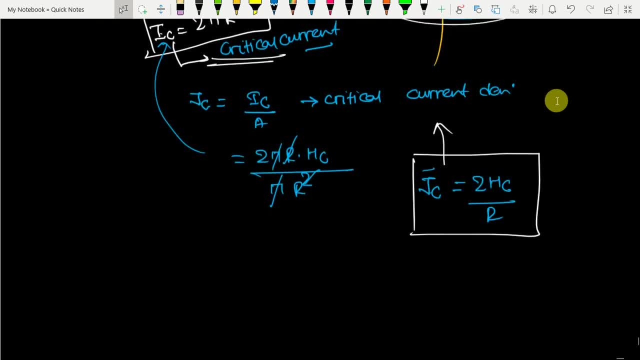 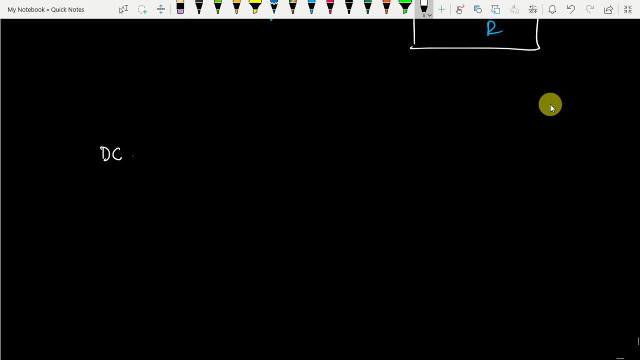 of this, superconductivity vanishes in this. in the case of that spaceman which we have taken now, superconductivity is mainly observed for dc and up to radio frequencies. you have to remember, because you can expect question later to this point: either for dc it will be visible, or for radio. 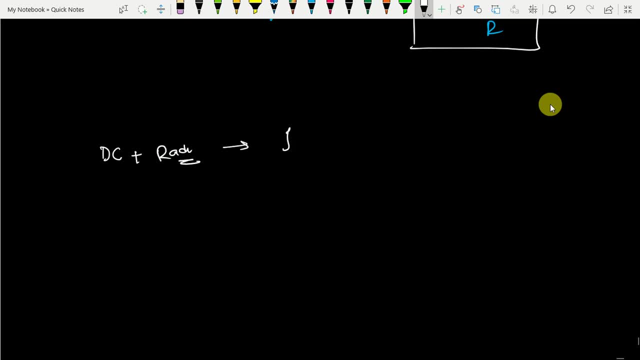 frequencies. if you will go to high frequency, high frequency will not be visible. superconductivity now the next point is super cooled coils. to understand what do you mean by super cooled coils? super cooled coils are such electric charges systems which can produce a flux density of 10 tesla or more in 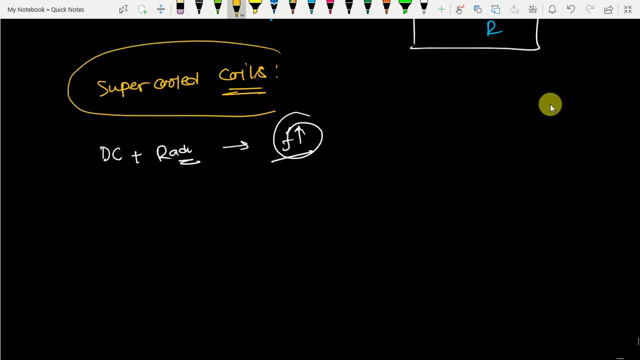 superconducting state. this is very much important because, as a design engineer, we need some devices which can produce us more and more magnetic field. so super cool coil kia hoga ki certain, under certain conditions. super cooled coils are those coils affiliate of an electrical system which can produce a flux density that is b. 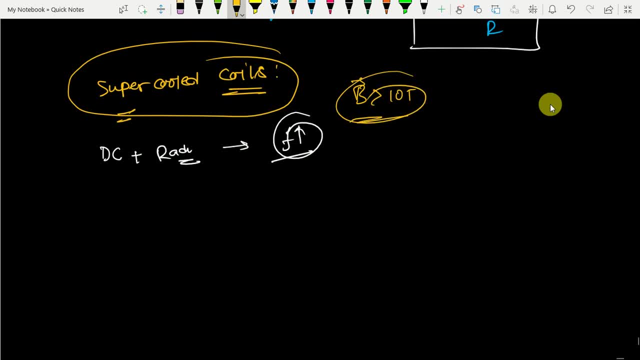 more than 10 tesla, which is very high, so it is very critical. temperature also varies with with relations to isotopic isotopes mass, that is, mass of an isotope. so you can say that you need not to go through in depth. you have to just remember that pc, that is, the critical temperature, is inversely proportional to root of. 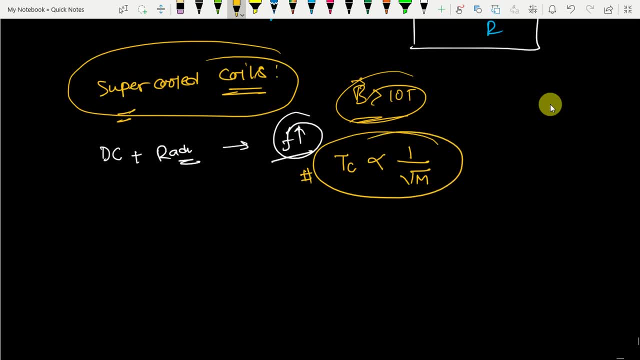 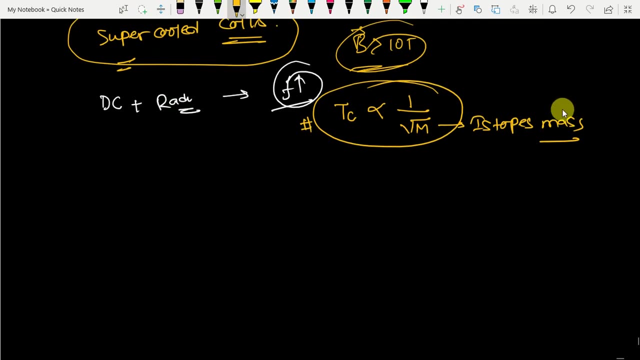 mass of an isotope. just remember this. you can also expect question related to this isotopes mass. now, up to here is conductivity, superconductivity. now let's move further to types of superconductivity. so types, kaka types in here don't get. first is type 1, super. 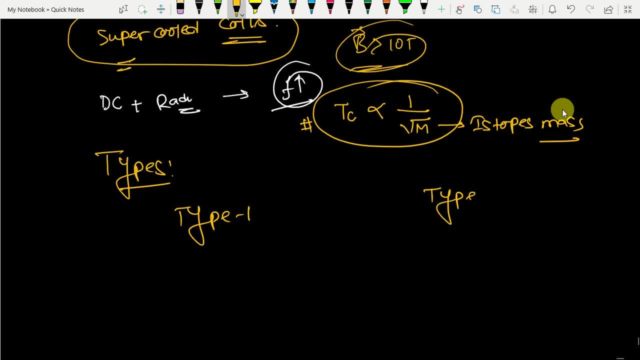 conductivity: type 1 superconductivity. second is type 2 superconductivity. type 1 superconductivity is also known as ideal superconductivity. this is ideal super conductivity and type 2 superconductivity is non-ideal superconductivity. now discussing about type 1. 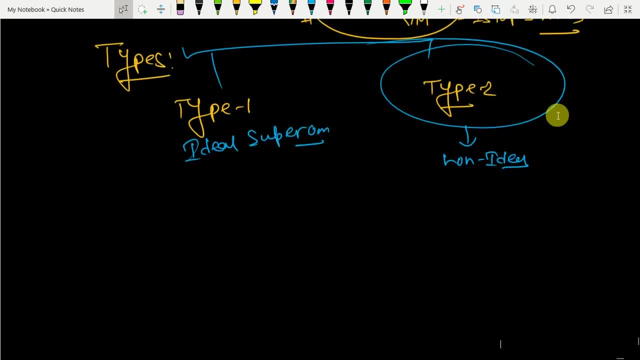 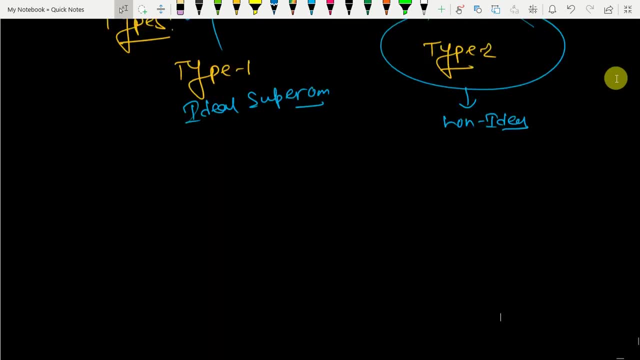 superconductivity and then after then, we will move up to type 2. now wait for a minute. now. type 1 superconductivity, type 1 or ideal superconductivity. you can say that in case of ideal superconductor or type 1 superconductor, these are soft superconductors. they have low value of critical magnetic field, that is, the hc value will be less low, very low in case of type 1 superconductor, or you can say that, ideal superconductors. the change of state from superconducting to normal and vice versa, exactly. 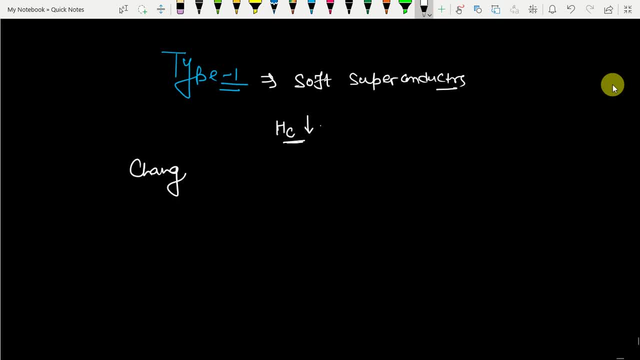 abrupt. that is the change of state. the change of state from superconducting to normal will be very abrupt and very fast. They exhibit complete Misenar effect and Silsby effect. Those type 1 superconductors will follow Misenar effect and Silsby effect completely. 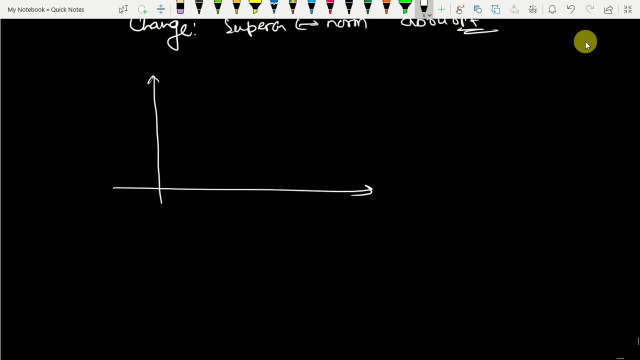 So you can see that. Now let me draw the graph between the magnetic moment M and the intensity H. So in case of type 1 semiconductor it is very abrupt. So you can see that like this, It is like this. This is at: h equals to hc. 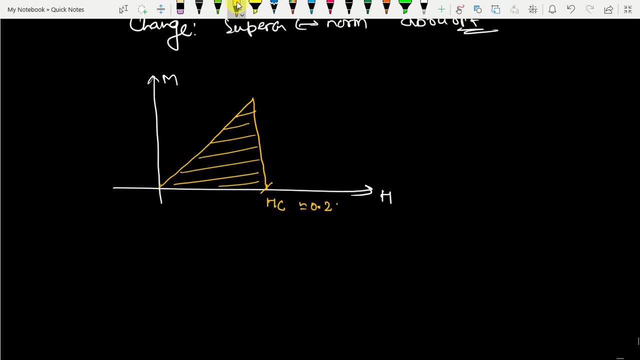 That is the critical intensity. Its value is nearly equal to 0.2 Tesla. as it is a soft superconductor, That is the ideal superconductor. This is the superconductivity space. That is superconductivity state and this is normal state. 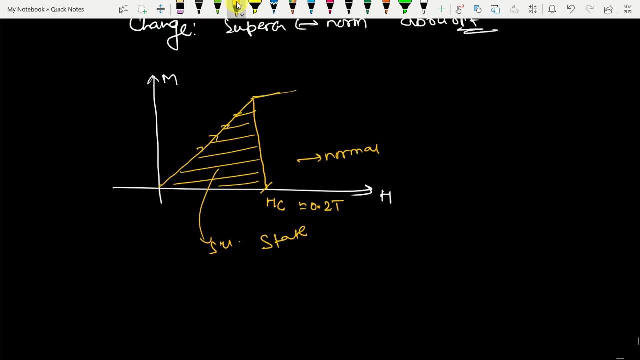 This is the abrupt change, Like if we are moving like this and suddenly we have to go like this. This is the abrupt city. Now let me move towards the type 2 semiconductor. What else do we call type 2 semiconductors? 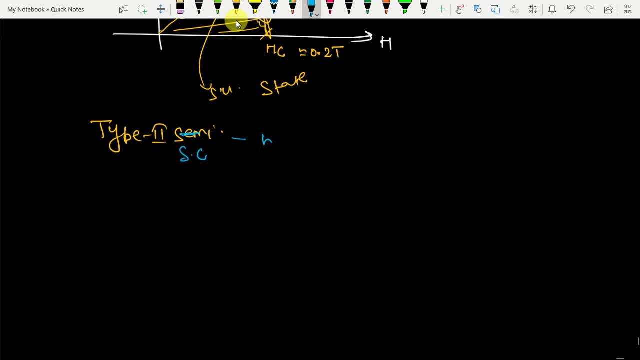 Non ideal, Sorry, type 2 superconductor, That is, non ideal superconductors. Now, non-ideal superconductors are also known as hard conductors. Let me move towards the type 2 semiconductor. So these are the non-ideal superconductors. 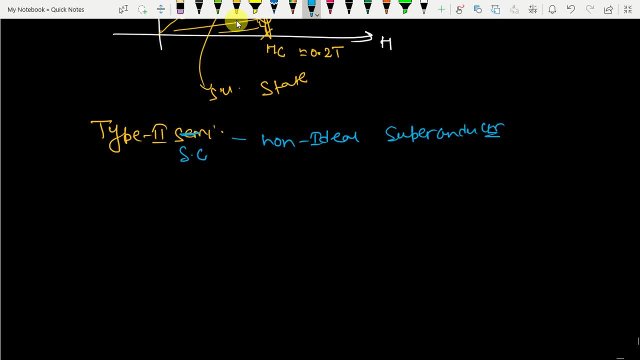 These are the non-ideal superconductors. they have high value of critical magnetic field. what will happen here? HC, that is, the value of critical magnetic field, will be high and transition temperature, TC, will also be high. the change of state from superconducting to normal and vice versa is graded. 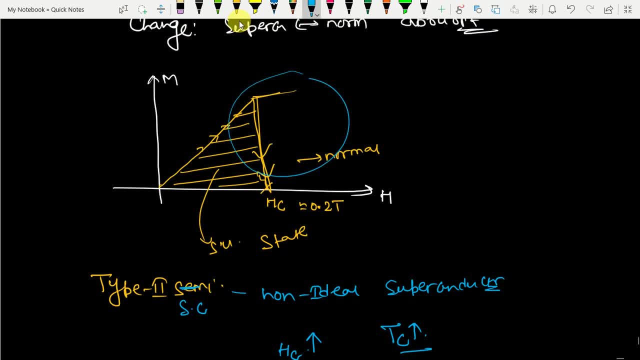 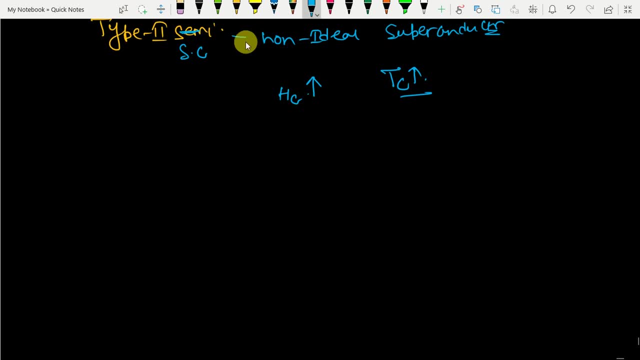 here the change in state, that is in case of type 1 superconductor, is abrupt change. but in case of type 2 superconductor the change in the state from superconducting state to the normal state is graded. that is slow. you can say that in case of type 1. 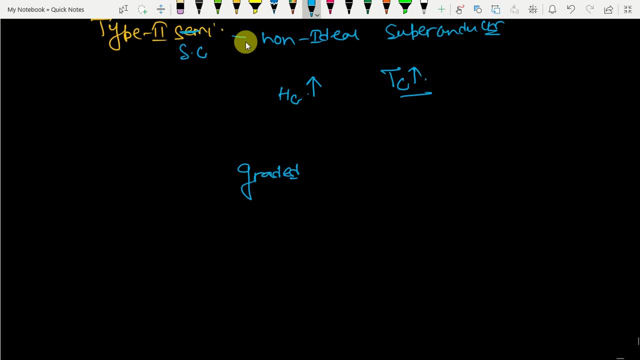 semiconductor. what we have expected is that the change in the state from superconducting to the normal state is abrupt and in type 2 superconductor the change in the state from superconducting material to the normal state is graded. they exhibit incomplete mizuner effect. first case: 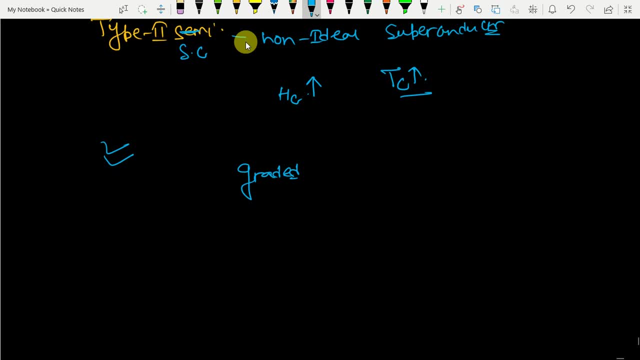 that is, type 1 superconductor exhibits complete mizuner effect and sils b effect, but in case of type 2 superconductor they effect incomplete mizuner effect and sils b effect. you need to remember this now. there are some. 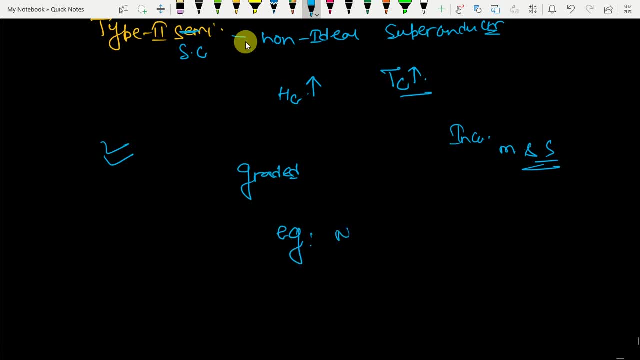 examples of type 2 superconductor: NBTI, NBZNZ, NB3SN, ATC. now let me show you the plot for type 2 semiconductor because engineering services UPC can ask you question related to curve. so this curve will be like this: 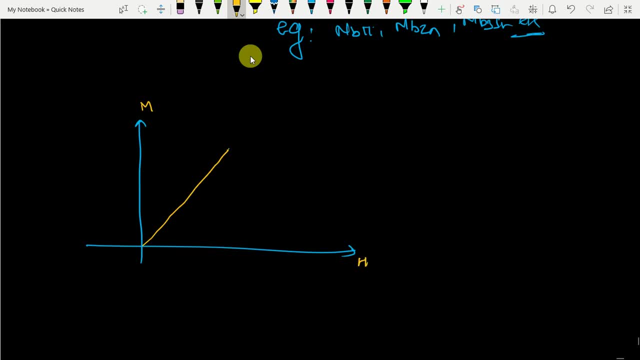 I am drawing the curve between m and h and after that it will be like this: that is graded portion. I am drawing this m versus h. so this is hc1, that is the critical temperature 1 and this is the hc2. this is the superconducting state. 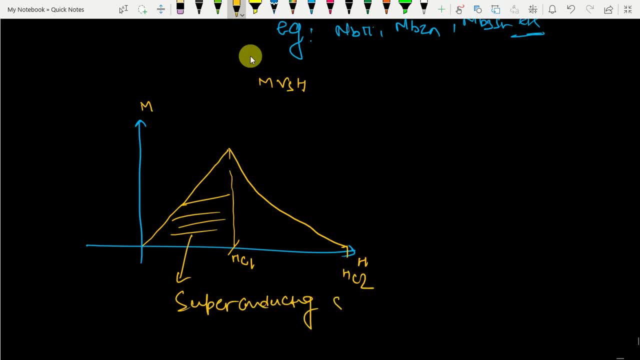 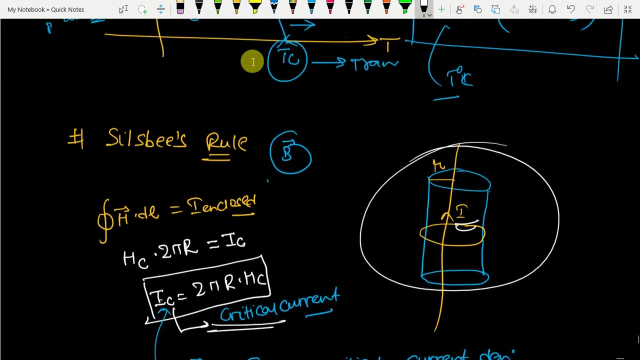 the state between hc1 and hc2. that is, the state between hc1 and hc2 is known as intermediate or vortex region, and after that it is normal region. so this is all about superconductivity and superconducting types of superconductivity and how you can. 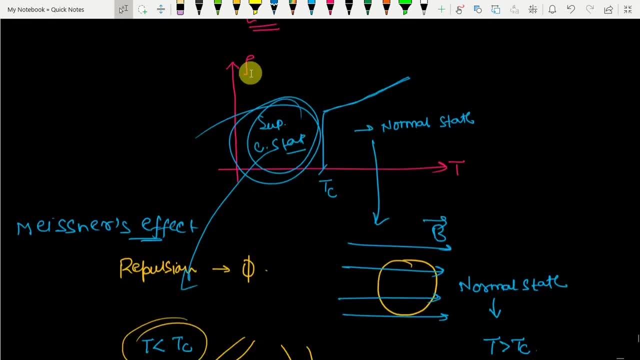 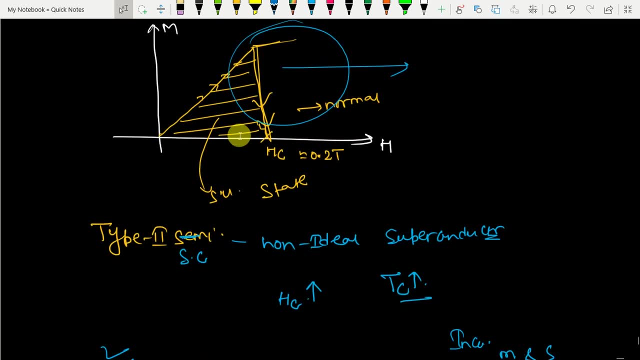 change the superconducting material to a normal material. so I am wrapping up right now and few more lectures. I will give you pdf of entire notes which I have prepared by using SP Seth and WD Callister. I will upload the entire notes of mine in my 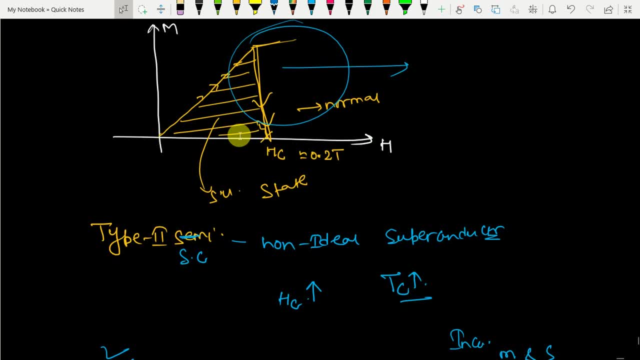 either on my facebook group channel that is gts simplified, or I will upload it in my telegram channel app. so stay tuned. thank you so much, wrapping up. 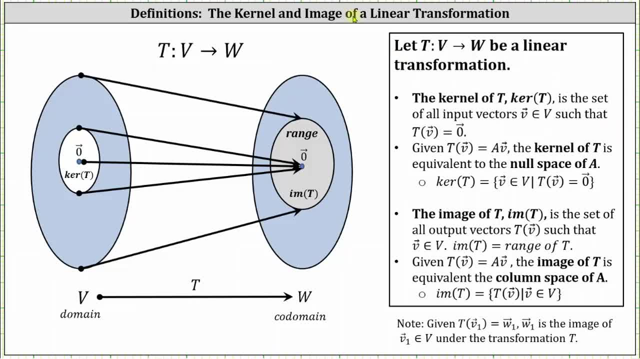 Welcome to an introduction to the definitions of the kernel and image of a linear transformation. Let the transformation t be from vector space v to vector space w be linear transformation, Then the kernel of t, denoted cur t, is a set of all input vectors v in the vector space v. 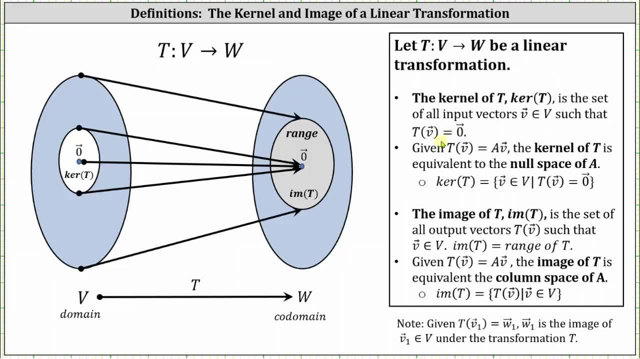 such that t of vector v equals the zero vector. And if we're given t of vector v equals matrix a times vector v, then the kernel of t is equivalent to the null space of matrix a. We can also state the definition of the kernel of t as shown here below. 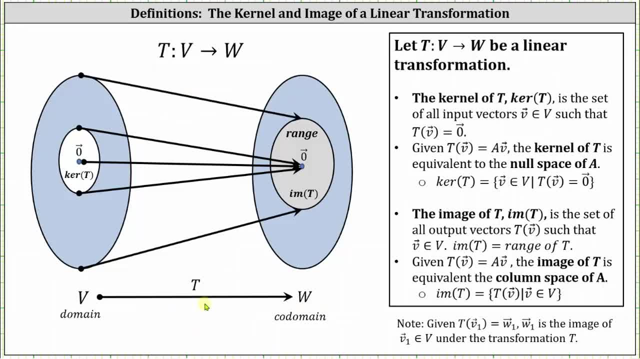 Take a look at the mapping on the left, Because we have a linear transformation from v to w. we know the zero vector in the domain maps to the zero vector in the range or set of outputs. But the kernel of t is a set of all vectors in the domain or the subset of vectors in the domain. 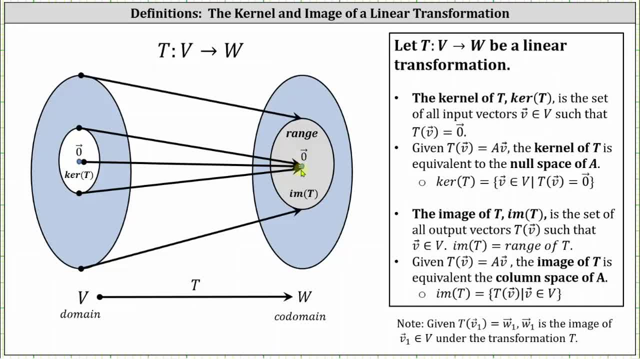 where the output is equal to the zero vector in the range. The image of t denoted mt, is a set of all output vectors, t of vector v, such that the vector v is in the vector space v or the domain, and therefore the image of t is equal to the range of t. 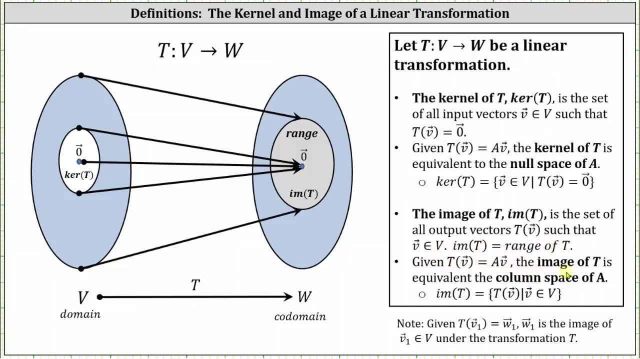 Given t, vector v equals matrix a times vector v. the image of t is equivalent to the column space of matrix a, And the definition of the image of t can also be stated using the notation shown here below. Going back to the mapping Again, the image of t is a set of all output vectors, t of